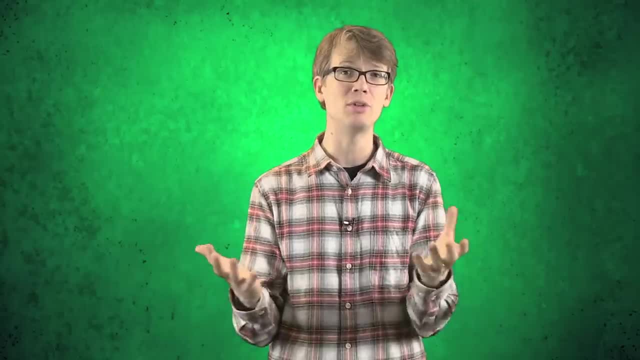 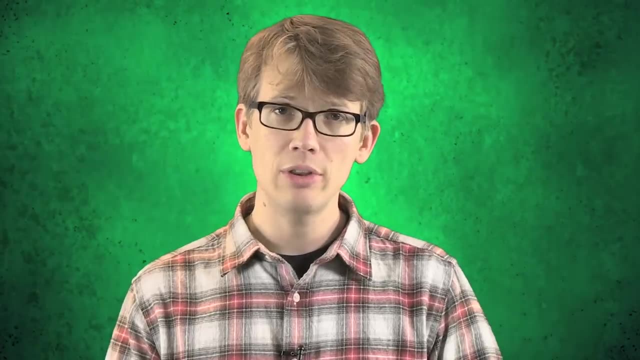 He became the first to demonstrate in a laboratory setting what Isaac Newton had been telling the world all along: that even small masses exert gravitational force on one another. The instrument he used to do this was complicated, but the principle behind it was pretty simple: A wooden rod. 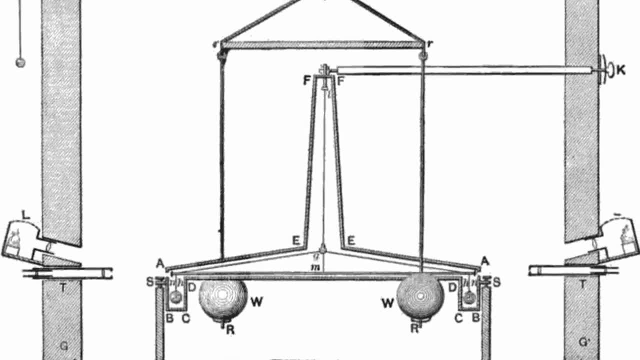 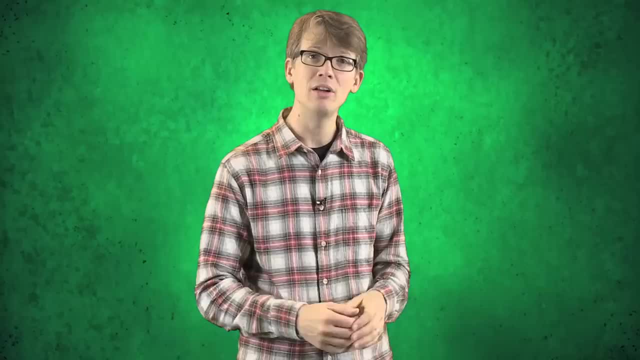 suspended from a wire with a small lead ball on either end, about three-quarters of a kilogram each. Then, near each small sphere, he mounted a much larger, 158 kilogram ball. Now, gradually but measurably, the gravitational attraction between the bodies. 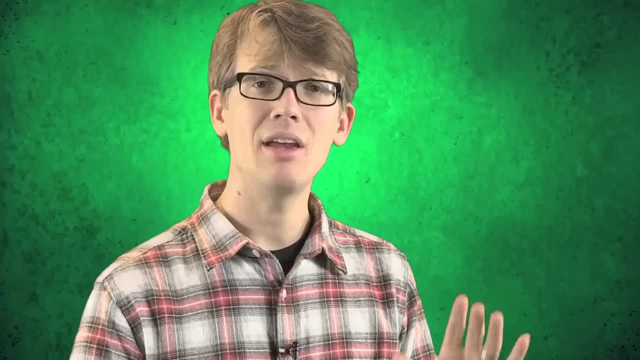 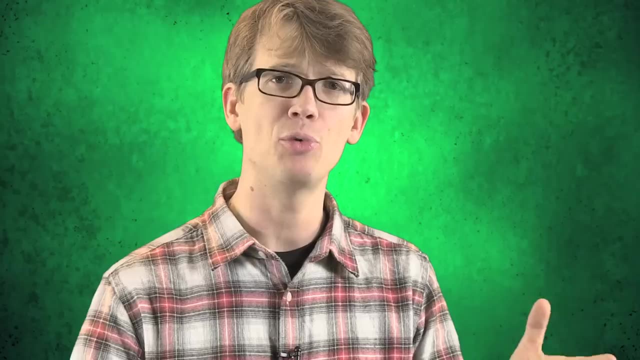 caused the small balls to move toward the big ones. In addition to demonstrating gravitation between objects, the results allowed Cavendish to actually measure it for the first time, by determining how much the rod moved and how much force was exerted on the wire as it twisted. 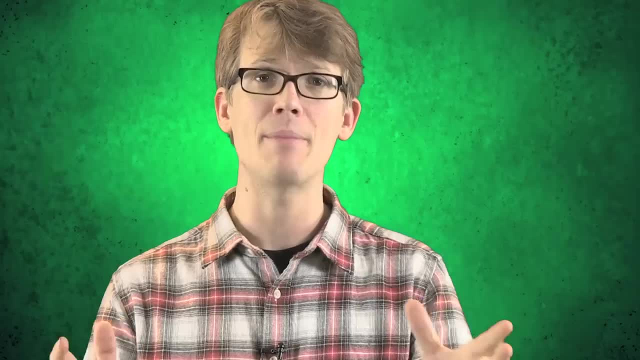 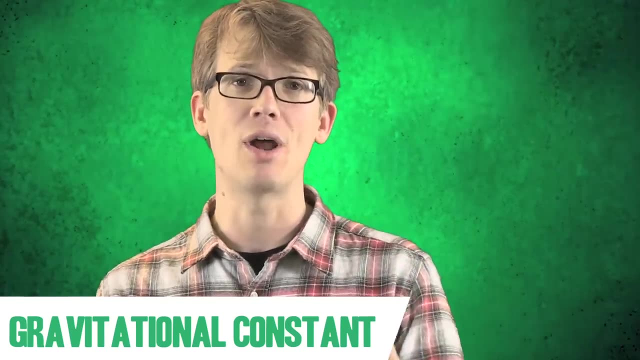 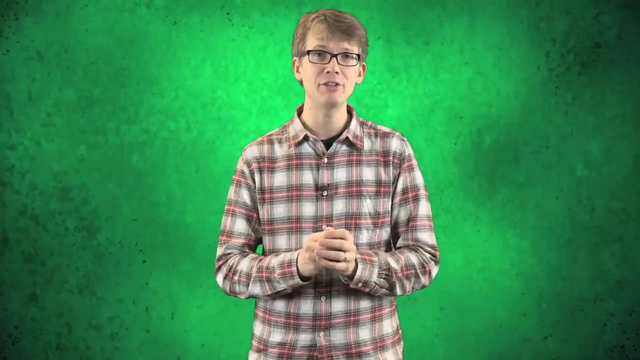 From this he was able to extrapolate all kinds of things. Perhaps most importantly, though, is what's now known as the gravitational constant, the figure that's actually used to calculate the gravitational force between any two objects. Number two: Thomas Young, makes waves. Less than 20 years after Cavendish, another gifted Brit, Thomas Young, revolutionized how we think about light. 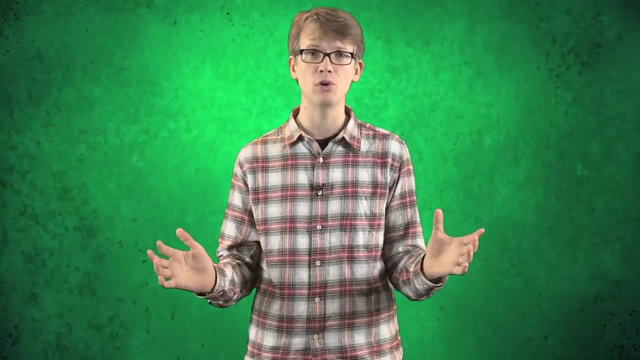 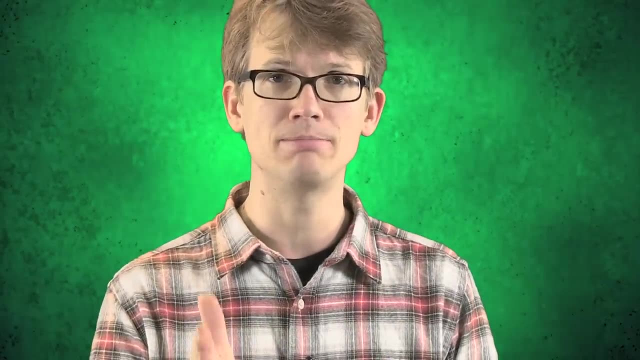 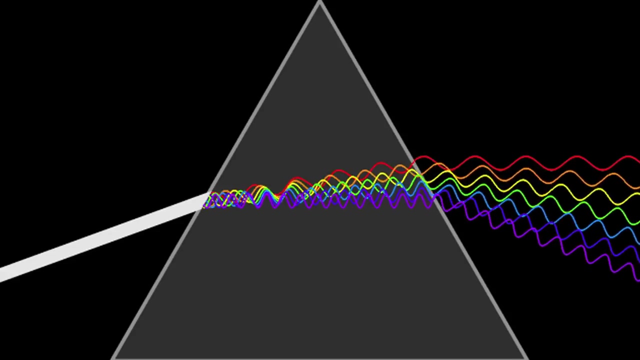 with an experiment that today is repeated in classrooms the world over. Back then, physicists were puzzling over how light moved as a wave, like sound does, or as a beam of particles, like Newton argued. Young thought Newton's particle theory didn't explain much of light's behavior, like how it refracts through a prism or the atmosphere. 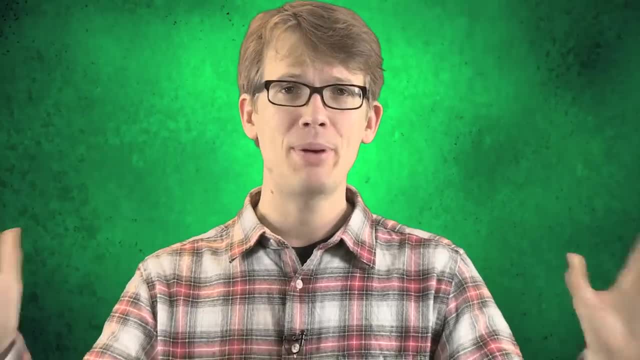 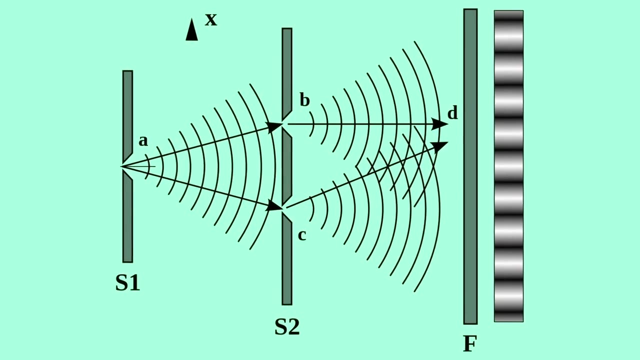 so he wanted to put the particle theory to the test. He covered a window with paper and then poked a small hole in it. He then bounced the beam of light that came through that hole onto a mirror and then held a thin card up to it. 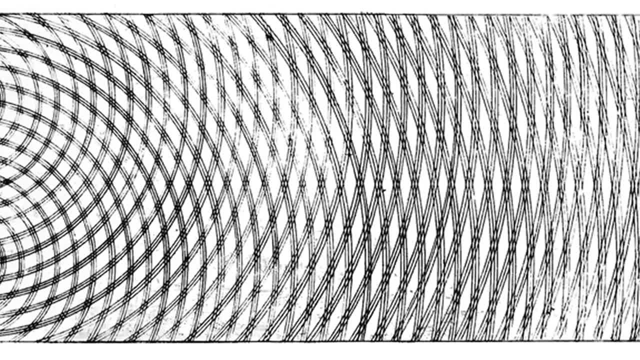 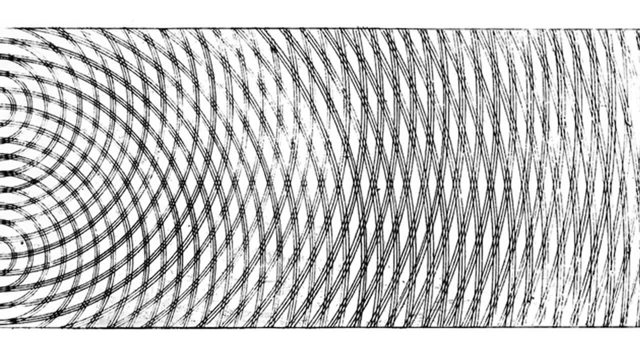 edgewise, which diverted the beam in And on the wall. the beams projected alternating bands of light that looked a lot like the pattern made when waves of water meet, with bright bands where the crests of two light waves crossed over, and dark bands where the crests from one beam met the trough of another. 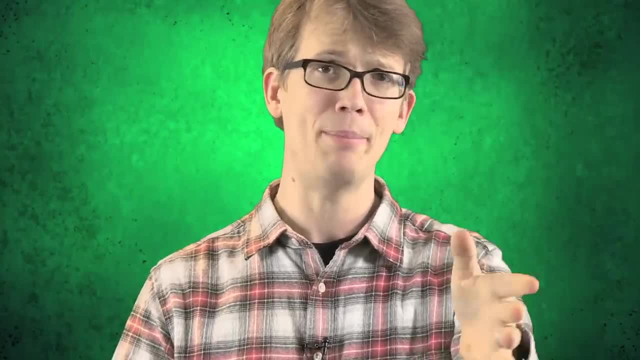 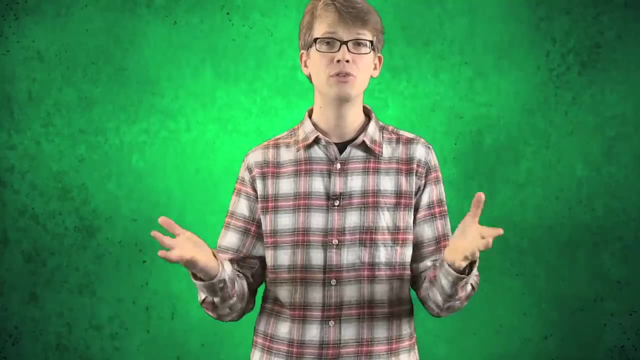 When Young shared his findings, physicists all over the world were dropping their monocles into their gin glasses, because contradicting Newton was pretty much like mooning the Royal Academy. The results showed that light, of course, did have wave-like properties, launching a scientific debate. 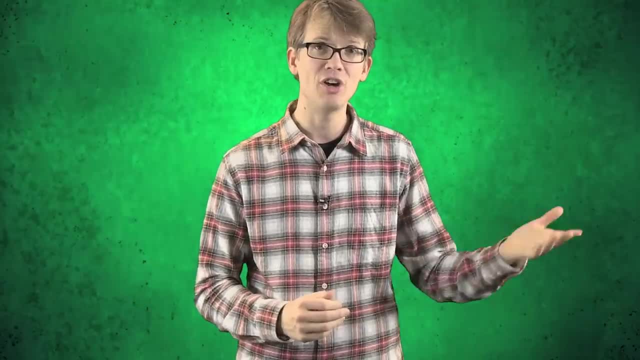 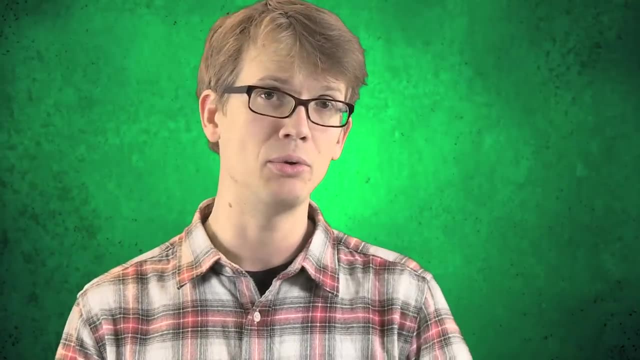 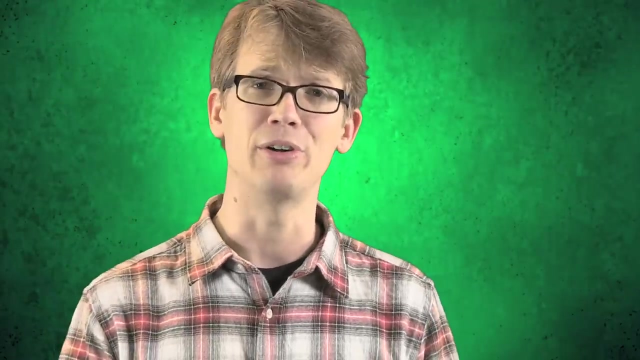 that would last nearly two hundred years, in which Young's experiment would be endlessly repeated, refined and built upon. In the end, though, it turned out that both Young and Newton were wrong, and also they were right. Today, quantum theory posits that all particles exhibit the properties of both particles and waves, a condition known as wave-particle duality. 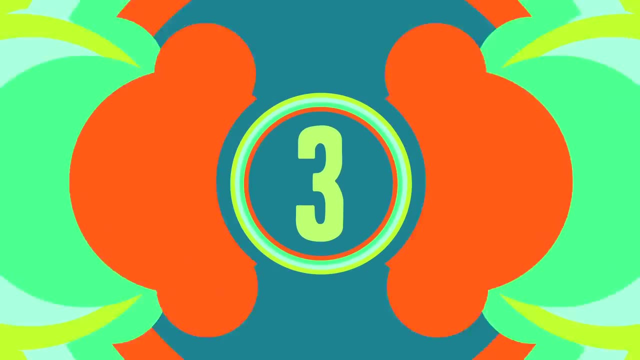 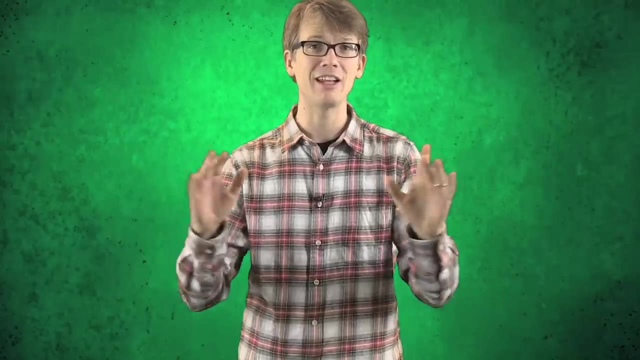 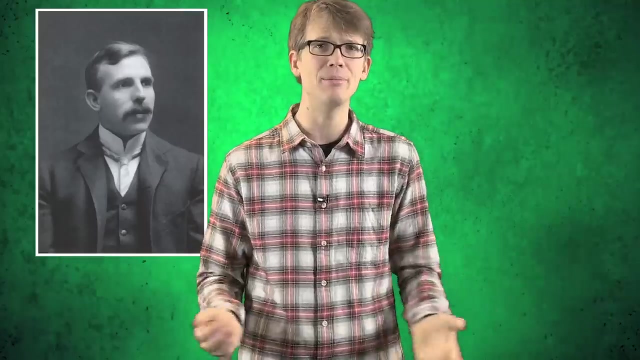 And that in physics is what we call a win-win And experiment. number three: Ernest Rutherford discovers that atoms aren't made of pudding. One of modern physics' most prolific and curious experimenters was Ernest Rutherford. His investigations led to the discovery of stuff like the half-life of elements and the existence of different kinds of radiation. 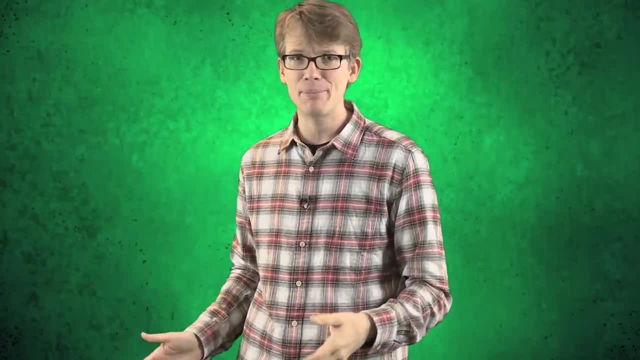 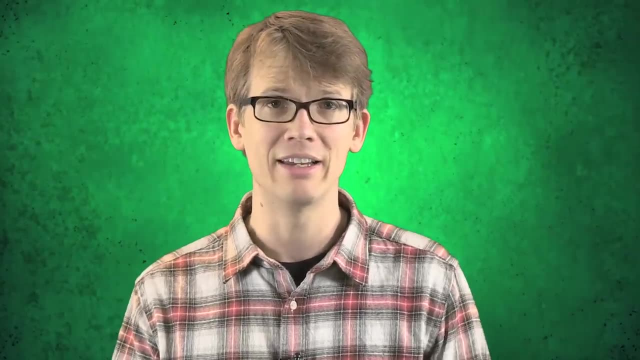 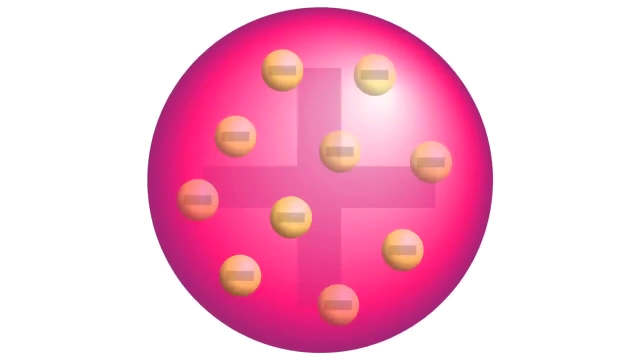 namely positively charged alpha particles and negative beta particles. But despite all of his intrepid research, by the early 1900s we still didn't know what an atom looked like. At the time, electrons had just been discovered and the prevailing theory was that they just floated around within a big positively charged 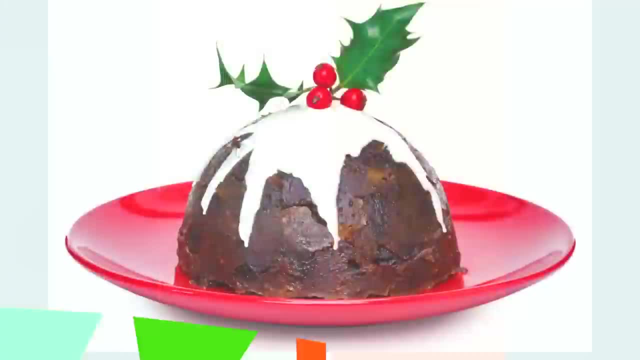 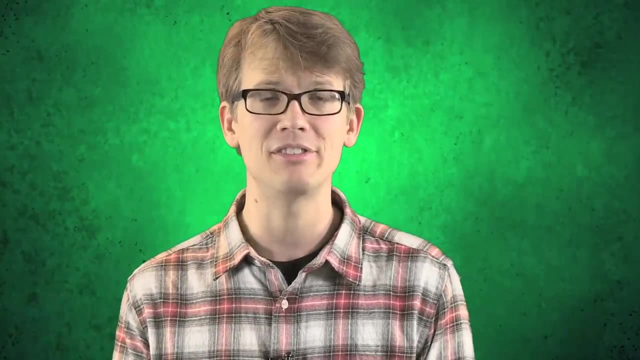 cluster of atoms, And that's what we're going to talk about in this video. And that's what we're going to talk about in this video. And that's what we're going to talk about in this video. This was known as the Plum Pudding Model- I'm not kidding- and while it sounded tasty, it didn't answer enough questions about the behavior of atoms to satisfy Rutherford. 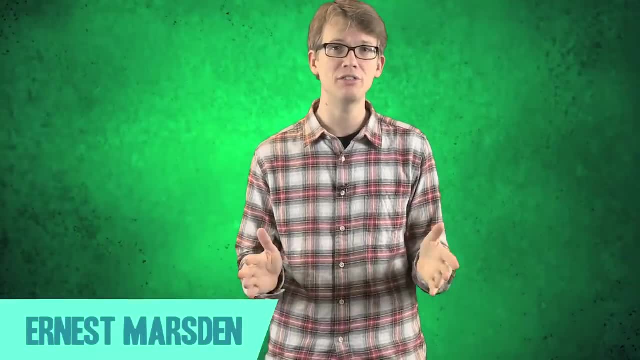 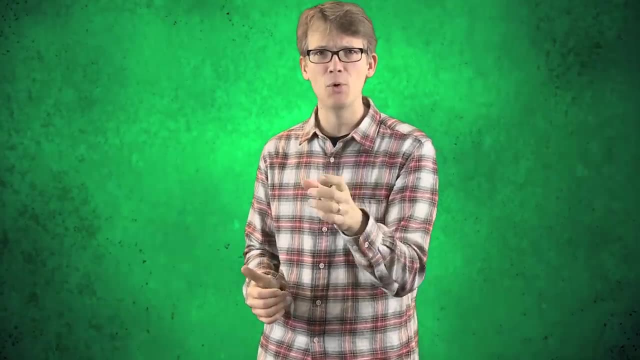 So in 1909, he and colleagues Hans Geiger and Ernest Marsden tested the theory. They aimed a beam of alpha particles at an infinitesimally thin foil of gold, a metal soft enough to compress into a layer just a few atoms thick. 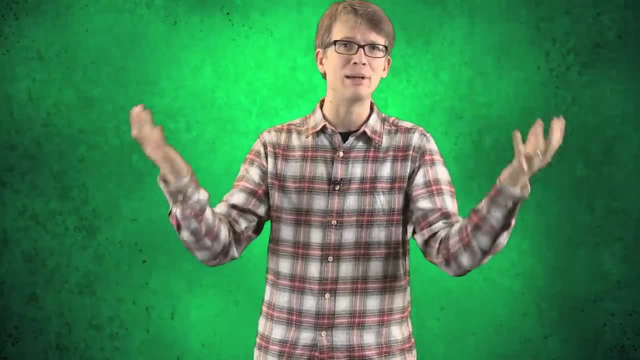 If the Plum Pudding Model was correct and atoms were just big, spacious clouds of foam. If the Plum Pudding Model was correct and atoms were just big, spacious clouds of foam, then alpha particles would pass right through the foil. 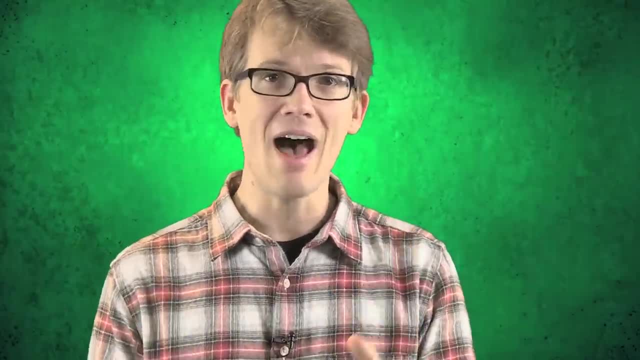 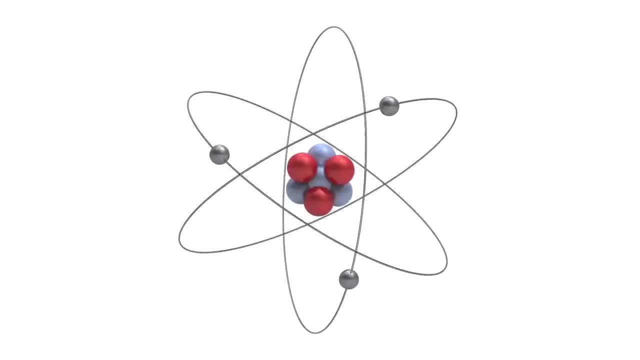 And interestingly, lots of them did, but many of them did not. They bounced off at sharp angles, sometimes flying right back at the source of the beam. Rutherford concluded that atoms must have a small, compact core, a nucleus with a net positive charge that deflected the alpha particles. 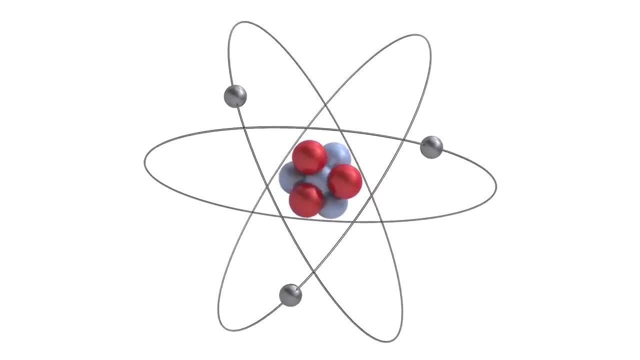 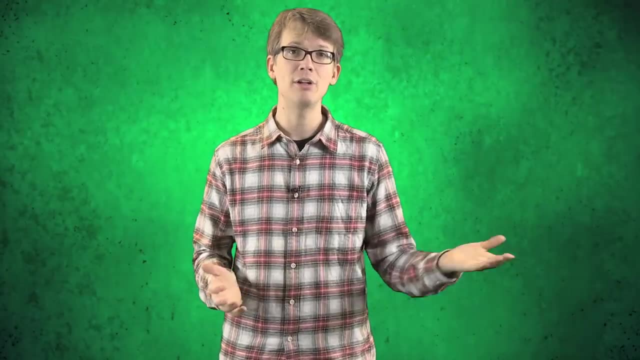 And rather than floating among the positively charged material, the electrons must be moving around it at a distance. This led directly to the atomic model that we know today, and its principles form the foundations of nuclear physics. Thank you for watching this episode of SciShow.